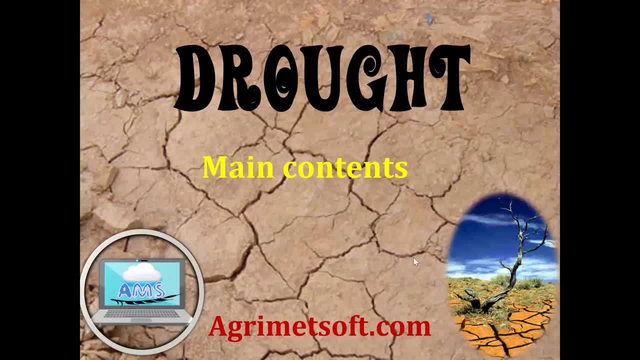 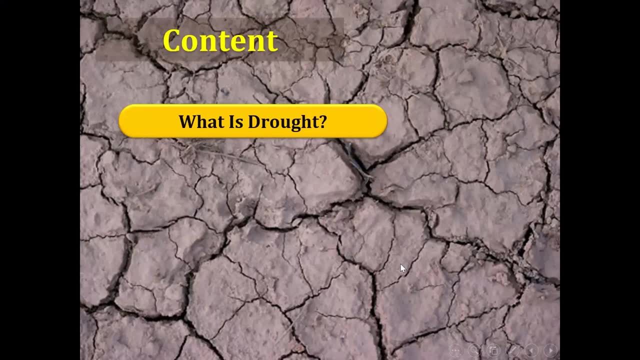 for you for knowing better drought and related concepts. Let's get started with the content You know. in the next videos we will focus on what is drought and what is the different definitions that we can focus and present them for drought according to literatures. 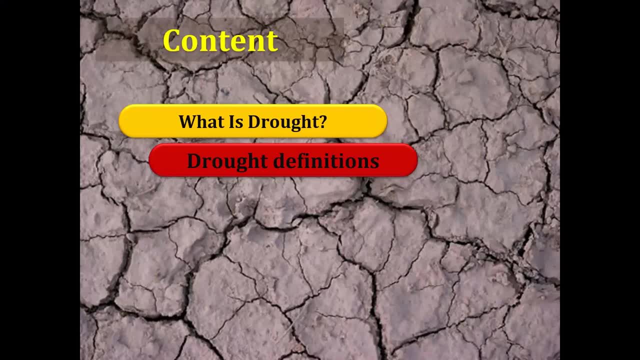 significant and critical literatures related to drought, And also we will focus on drought and aridity concept. We will try to present the definite definitions and differences between drought and also aridity. So then, after we will try to present you unique characteristics of drought, such as 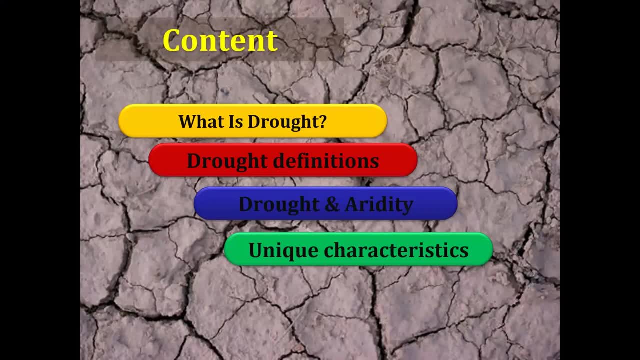 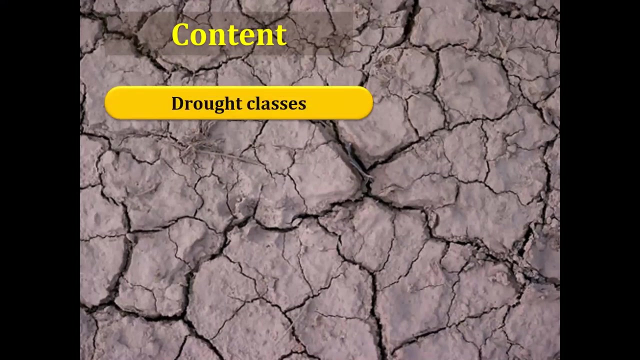 severity, such as I mean the frequency and period that drought would be happening, And then, after, we will try to search and find environmental factors and effective factors would be cause of the drought events. And, by the way, we will focus on drought classes. what can be categorized them? how can we categorize? 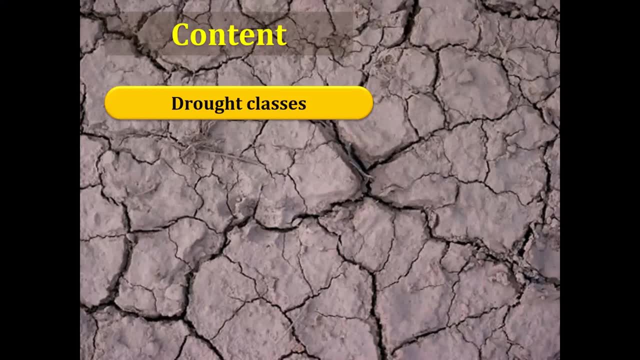 them and what are the main classes in drought events? Okay, Then after we will try to focus on drought indices. What are the most significant drought indices and when we call it, is a drought index in metrological index? I mean that and like that. what the main concept? 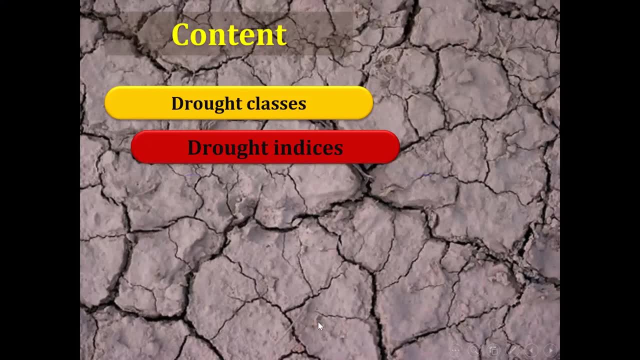 I will tell you how can we find them and how can we define them. And then, after it is so important for us As climatologists or metallurgists or agro-metrologists to calculate these indices. How can we calculate them? 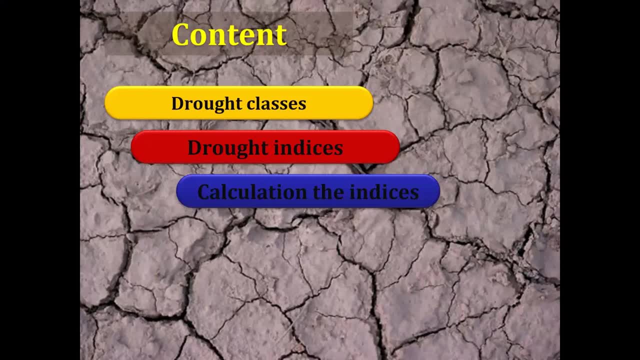 What are the fundamental literatures about calculating indices? I will share all of them with you And then, after I will introduce some useful tools for fluent them for you. How can we calculate these indices? which we? which one of the important tools? how? 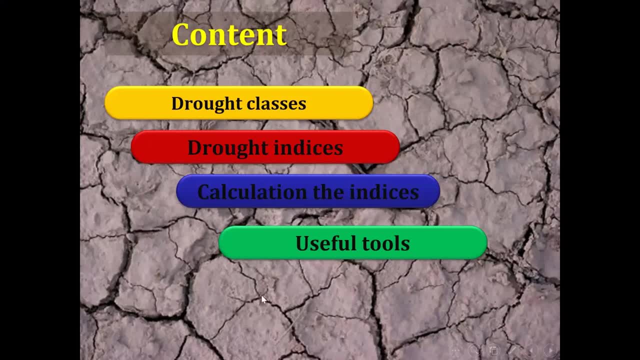 can we define them? Okay, How can we define them? And like that and so on, new concepts and projects are all around the world about drought and how can we define a new projects to get a job, or maybe get some proposal or define, submit some proposal? 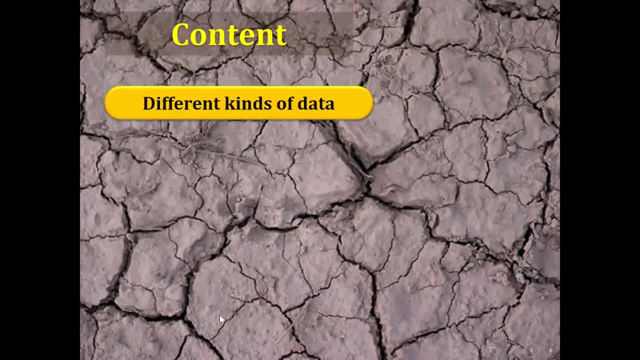 How can we do that? In the next step, we will try to use different kinds of data. I meant that as an answer to data. uh, can we do them? And what about gridded data set? How can we use them for monitoring drought and calculating drought events? different drought. 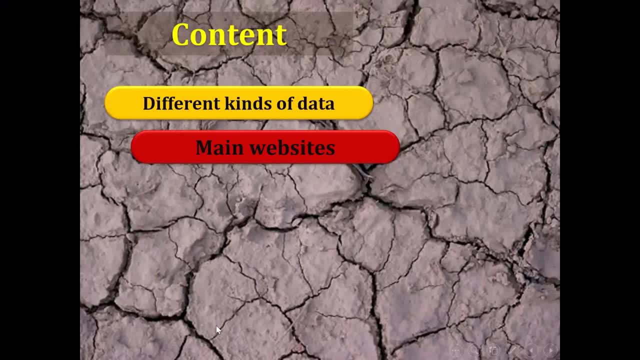 events. I mean that Then after I will try to introduce you main website, main effective website that would be a useful for you, applicable for you to better understanding different new uh cases or maybe news about drought. Then, after a bit, we'll try to focus on different significant papers. 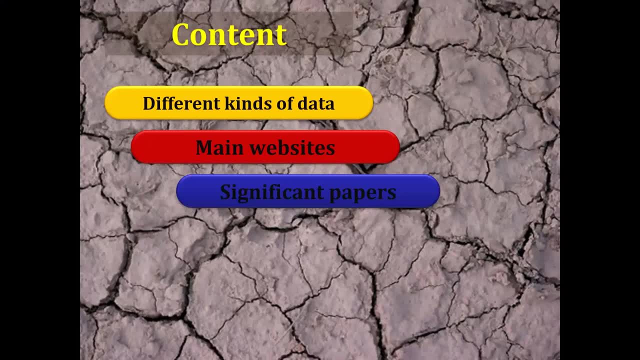 That's all of them. Okay, That would be helpful for us to better understanding and dominant on uh this uh effective. I mean that this uh hazardous event- drought- and then we will try to find the best papers. 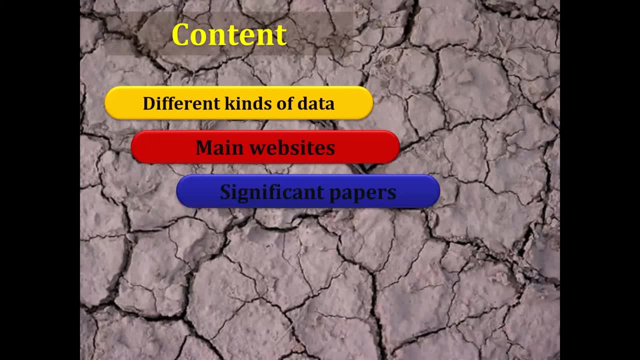 uh, trace them to find different indices, And we want to answer this question and address different gaps on them and like that. Then, after you know we have some uh methods or maybe it will be better to say that, Okay. 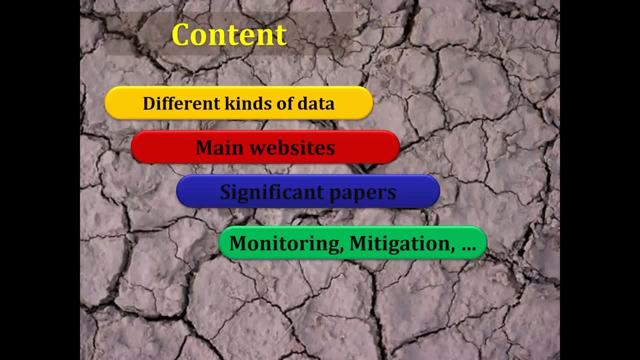 Okay, Okay, So that we have some process, uh to uh detect or recognizing drought, uh such as monitoring, mitigation or vulnerability and, finally, sustainability. In this series of video, I will try to show all of this content and I promise you I will. 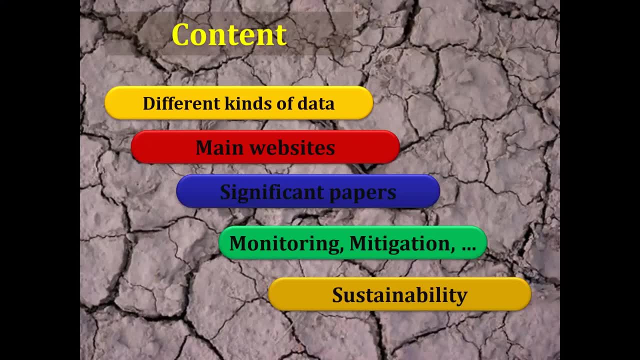 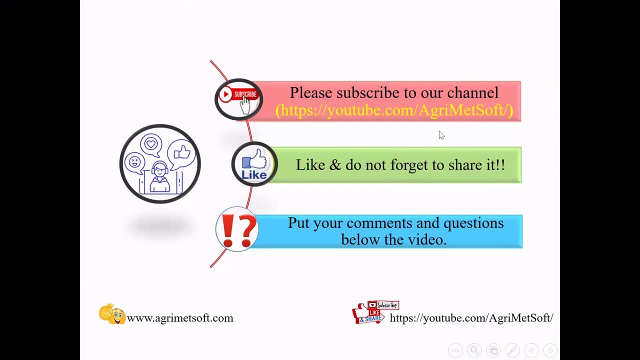 back soon and continue these series of videos as quickly as possible And at the end, Okay, Okay, channel with this address that you can see here. like, and don't forget to share it. put your comments and questions below this video and let me know your ideas. i mean that, what are the main ideas?